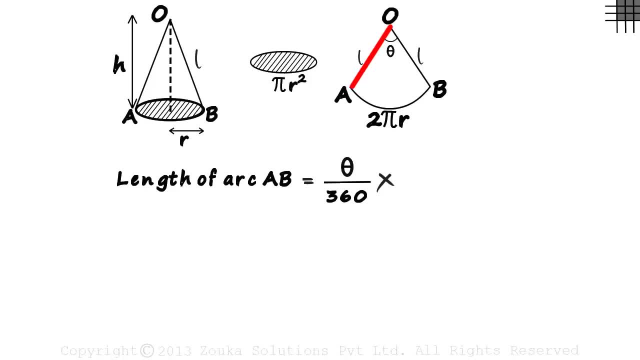 multiplied by the circumference of the circle, with radius OA and OB. What will be the circumference of the circle that is formed with this as the sector? It will be 2 pi L, since L is the radius of the circle of which this sector is a part. This tells us that the length of 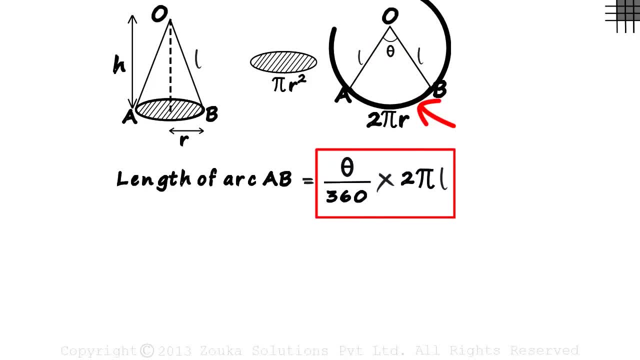 arc AB is a part of the circumference of the big circle that can be formed here. But the length of arc AB is also 2 pi R. That will equal theta by 360 multiplied by 2 pi L, Cancelling 2 pi out from both sides. 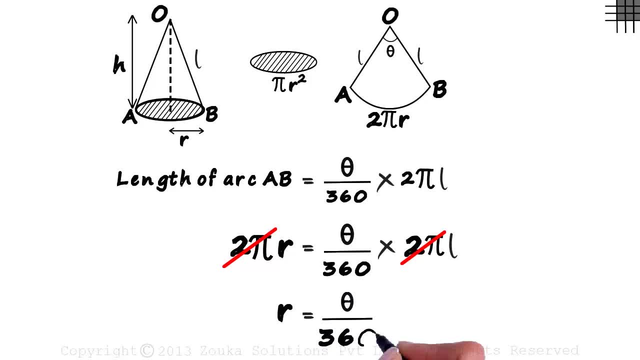 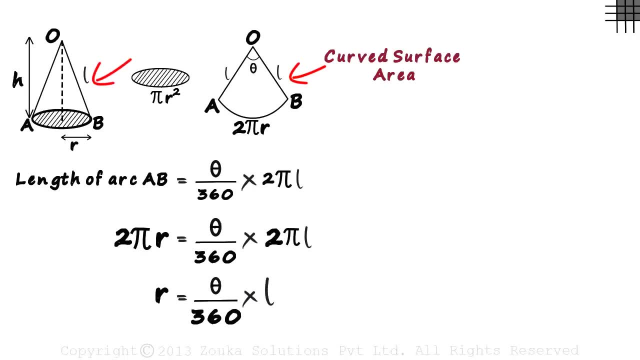 we get R equal to theta by 360 multiplied by L. The area of this sector will be the curved surface area of this cone. The area of this sector will equal theta by 360 multiplied by the area of this circle with OA and OB. 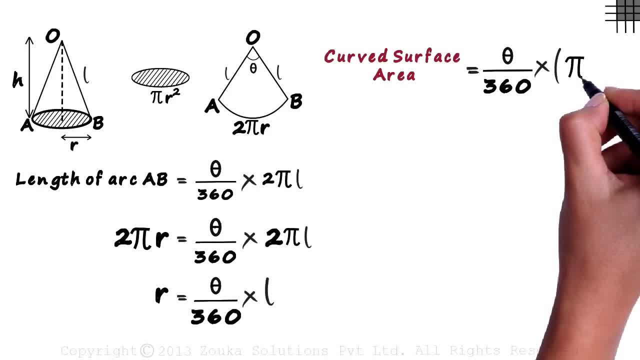 The area of this sector will be the curved surface area of this circle with OA and OB. The area of this sector will be the curved surface area of this circle with OA and OB. Can we write this a bit differently? Yes, this can also be written as pi L multiplied. 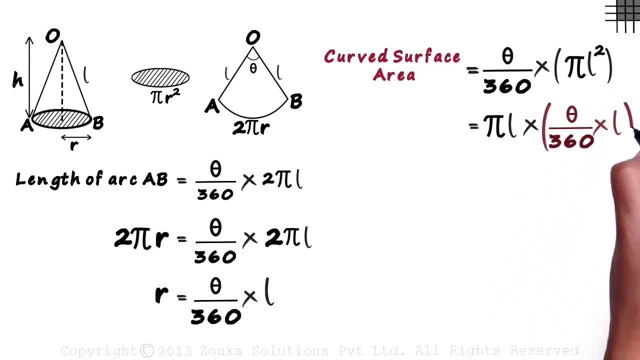 by theta by 360 multiplied by L. We have just split pi L squared into pi L multiplied by L, But this part in brackets, as we just found out, is equal to R, So the curved surface area will be pi L multiplied by R. 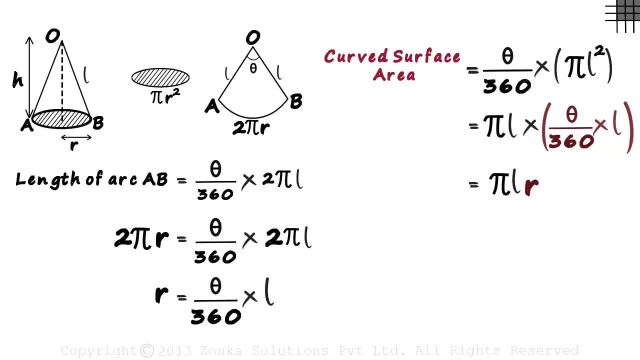 Let us review what we just did. We found out the length of arc AB in two different ways and equated them, And then we found out the curved surface area using the formula of a sector of a circle And then finally substituted the value of R in this formula to eliminate. 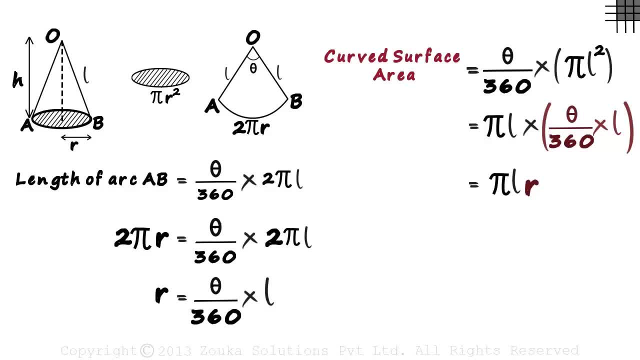 theta. Now it's very simple. The total surface area of the cone will be the curved surface area plus the area of the circular base. The curved surface area, as we know, is pi L R And the area of the base is pi R squared. 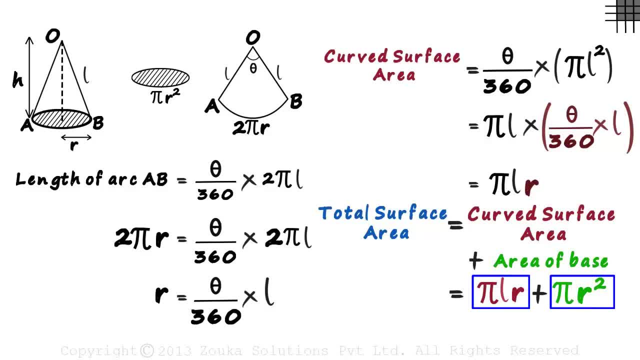 Both the terms have pi R as their common factor. Taking pi R common, we write the formula as pi R multiplied by L plus R. This is the formula for the total surface area of a right circular cone.